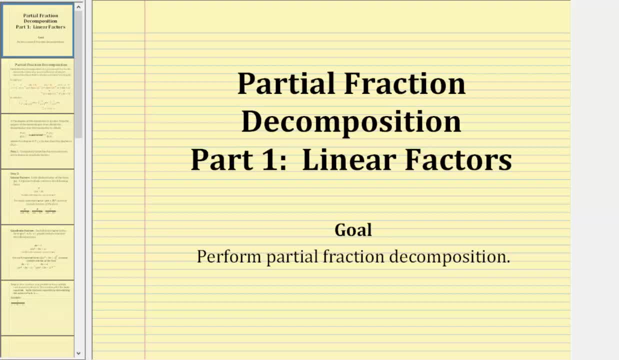 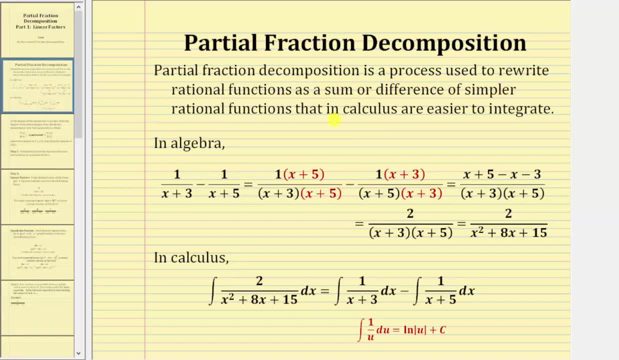 Welcome to part one of a lesson on partial fraction decomposition. Partial fraction decomposition is a process used to rewrite rational functions as a sum or difference of simpler rational functions which in calculus are easier to integrate. We know from algebra. we often add or subtract rational expressions by obtaining a common denominator and then adding or. 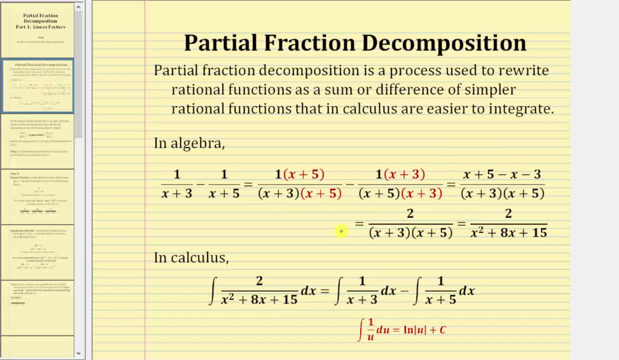 subtracting the numerators to write the sum or difference as a single rational expression. However, partial fraction decomposition is just the opposite of this process. For example, in calculus we may have a difficult time integrating a specific rational function because it does not fit a specific integration. 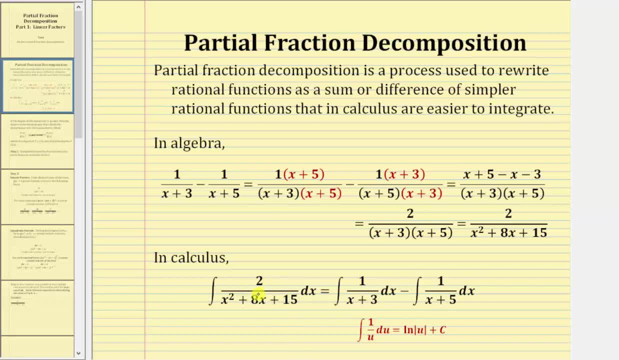 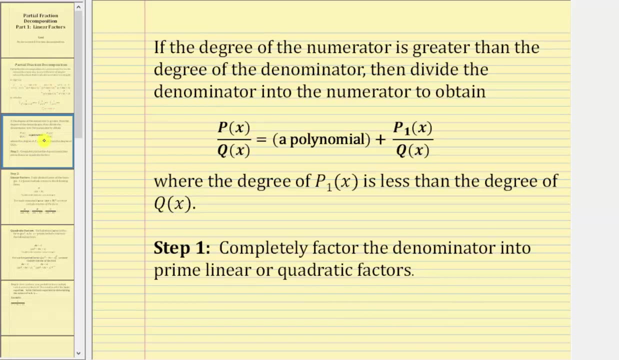 formula. However, we can sometimes write the rational function as a sum or difference of simpler rational functions which are easier to integrate, which is why the process of partial fraction decomposition can be very useful. However, before performing partial fraction decomposition, if the degree of the numerator is greater than the degree of 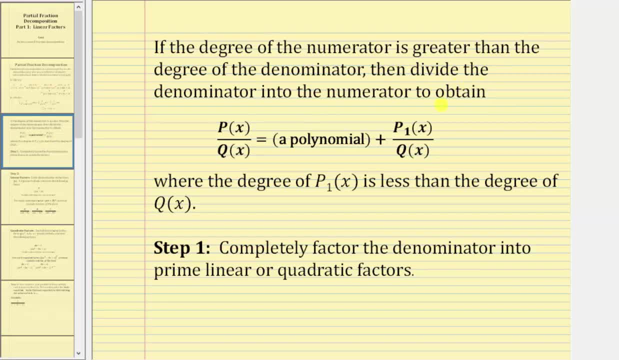 the denominator, then we must divide the denominator into the numerator to obtain a polynomial plus a rational function where the degree of the numerator, or P sub 1 of X, is less than the degree of the denominator, or in this case Q of X. Once we have the rational function in the correct form, the first 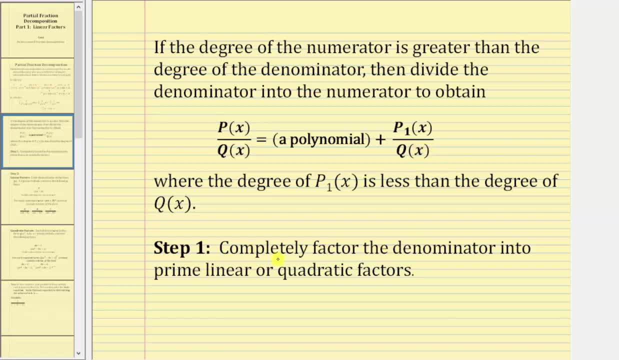 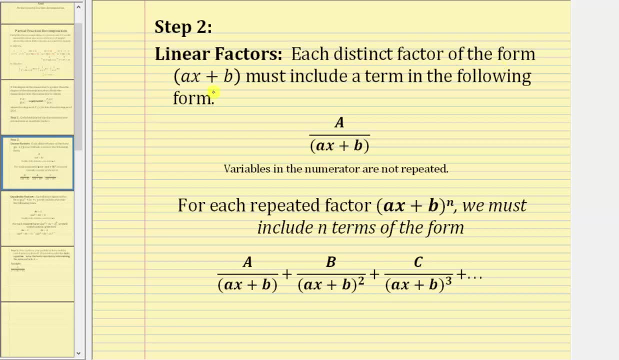 step is a completely factor of the denominator into prime, linear or quadratic factors. Step two: for linear factors, each distinct linear factor in the form ax plus b must include a term in the following form: where we have a single variable in the numerator and the variables in the numerator are not repeated. 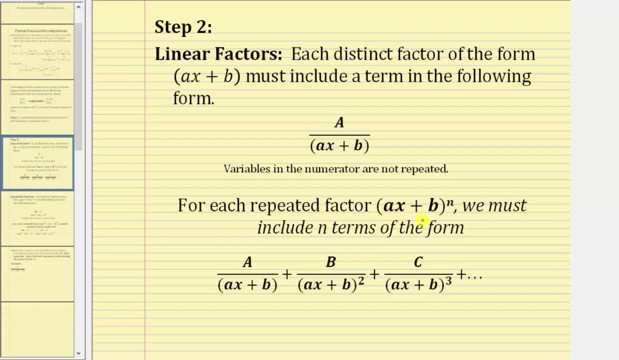 For each repeated linear factor in the form the quantity ax plus b raised to the power of n, we must include n terms of the following form: Again, notice how the variables in the numerator are never repeated For quadratic factors, each distinct quadratic factor. 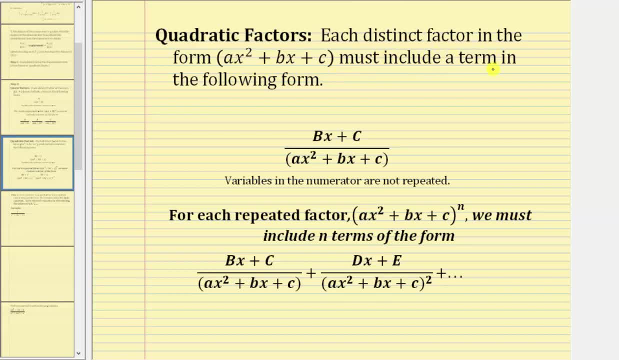 in the form ax squared plus bx plus c, must include a term in the following form where, notice now the numerator is a linear factor For repeated factors in quadratic form raised to the power of n. we must again include n terms of the following form and once again notice how the variables in the numerator 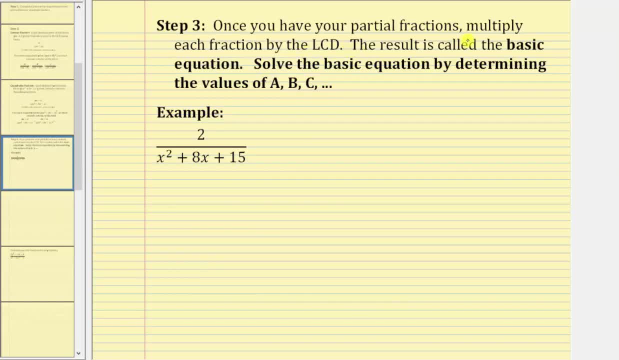 are never repeated. For step three, once we have the partial fractions, we multiply each fraction by the LCD, and the result is what's called the basic equation, which we then solve for a, b, c and so on. So let's perform partial fraction decomposition. 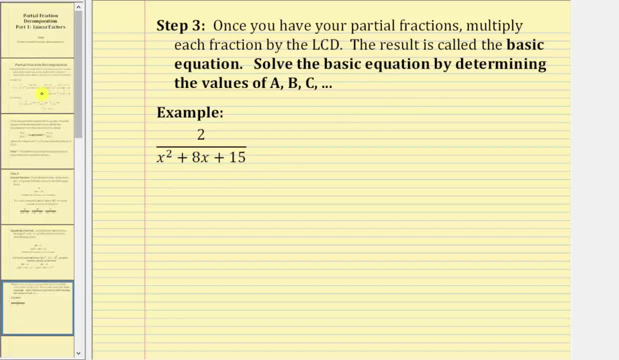 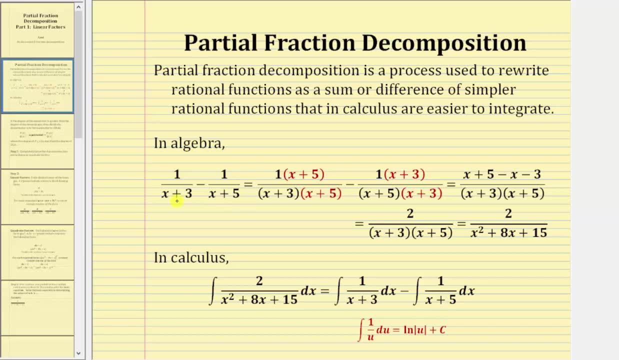 on this rational expression which we should remember from the first slide, should give us one divided by the quantity x plus three, minus one divided by the quantity x plus five, because we know the difference. is this rational expression here. Let's just verify: we get the same result. 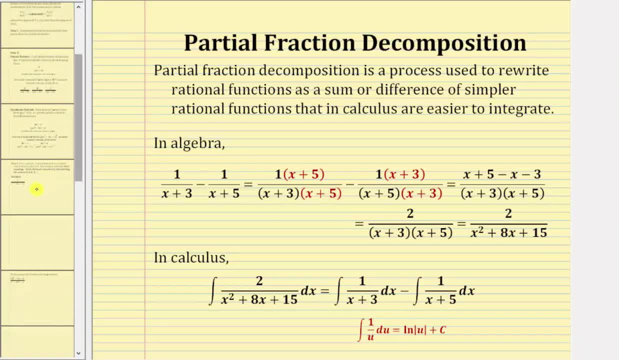 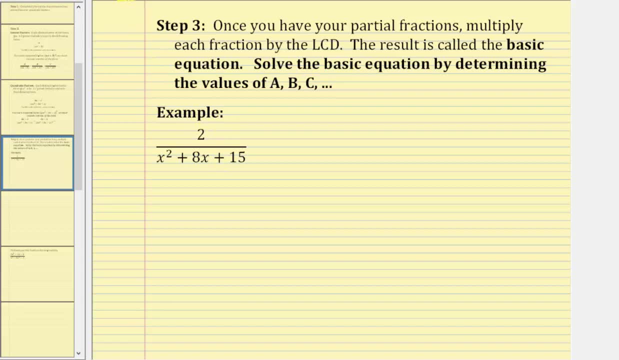 by performing partial fraction decomposition. So again, the first step is to recognize again that we get the same result by performing partial fraction decomposition, So we can recognize the degree of the numerator is less than the degree of the denominator and therefore we can go ahead and proceed. 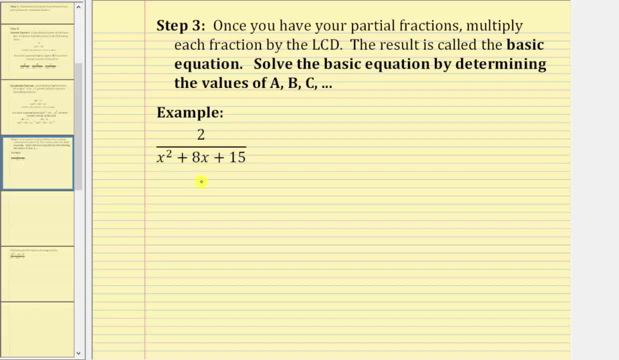 to partial fraction, decomposition and factor the denominator And the denominator factors into two linear factors. The factors of x squared are x and x. The factors of 15 that add to eight are positive three and positive five, which give us x plus three times x plus five. 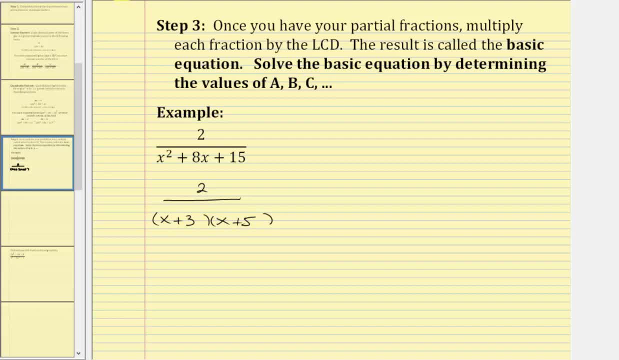 And now, because we have two distinct linear factors in the denominator, this rational expression is equal to a divided by the linear factor of x plus three, plus b divided by the linear factor of x plus five. Now, if we had a over x plus five and b over x plus three, 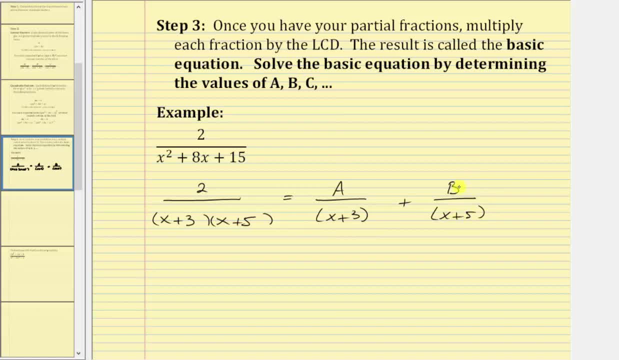 that would be just fine as well. The next step is to clear the fractions from the equation by multiplying both sides of the equation or each rational expression by the least common denominator, which is x plus three times x plus five. So let's go ahead and set that up. 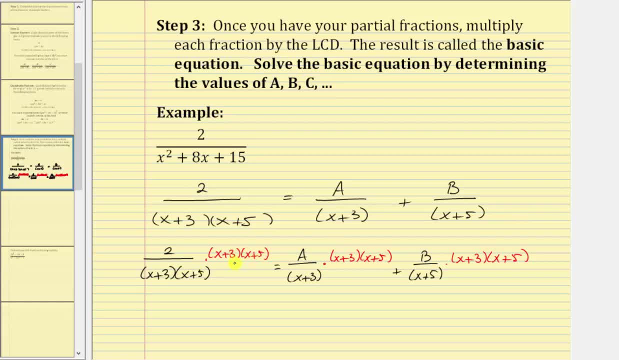 If it's helpful, we can write the factors of x plus three and x plus five as a fraction, with the denominator of one. And now, before multiplying, we will simplify out all the common factors between the numerators and denominators. Notice: here we have a common factor of x plus three. 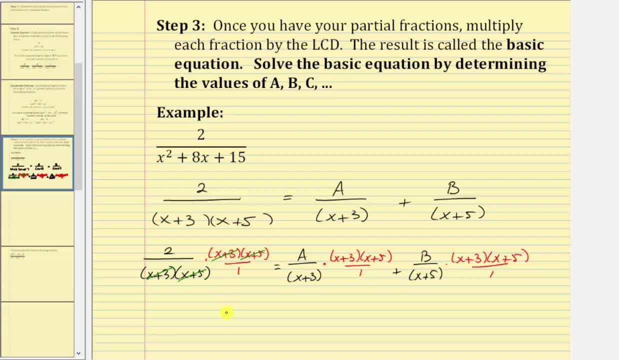 as well as a common factor of x plus five. We now just have two on the left, so we have two equals On the right side. a factor of x plus three simplifies out here, leaving us with a times the quantity x plus five. 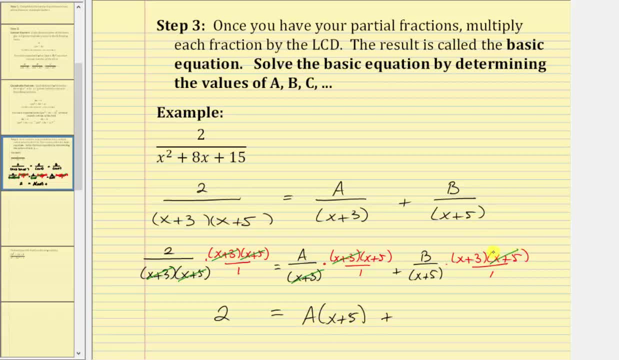 And then we have, plus here, a common factor of x plus five simplifies out, leaving us with b times the quantity x plus three. So this is our basic equation, which we now need to solve for a and b. Let's take this to the next slide. 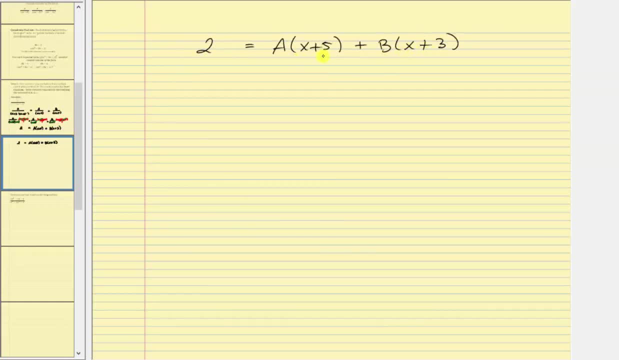 This equation is true for all values of x. however, if we select convenient values of x, it makes it much easier to solve for a and b. Notice how, if we let x equal negative five, x plus five would be zero. If we let x equal negative three. 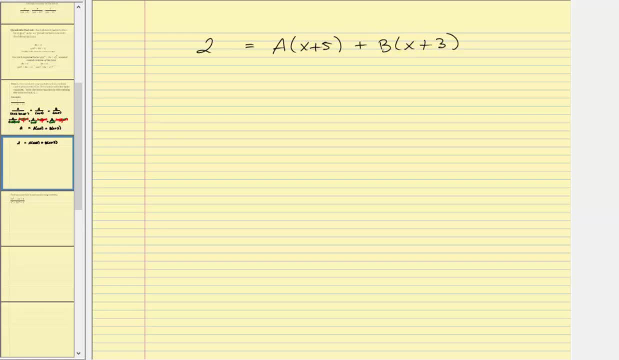 x plus three would be equal to zero. So let's begin by letting x equal negative five. If x is negative five, we have the equation two equals a times the quantity x plus five. But if we substitute negative five for x, we have negative five plus five, which is zero. 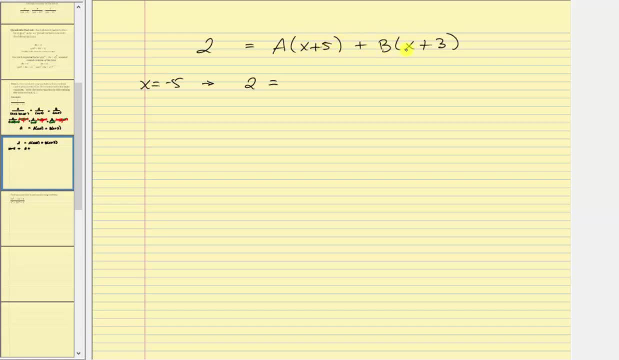 A times zero is zero. And then we have plus b times the quantity negative five plus three, which is b times negative two or negative two, b Solving for b: here we divide both sides by negative two, which gives us b equals negative one. 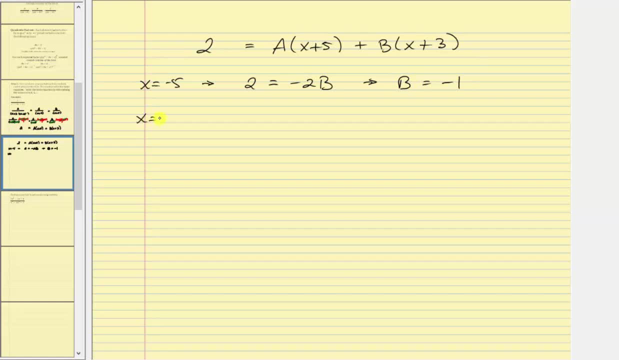 And now to solve for a. let's let x equal negative three. When x is negative three, we have the equation: two equals a times the quantity negative three plus five, which is a times two or two. a If x is negative three. 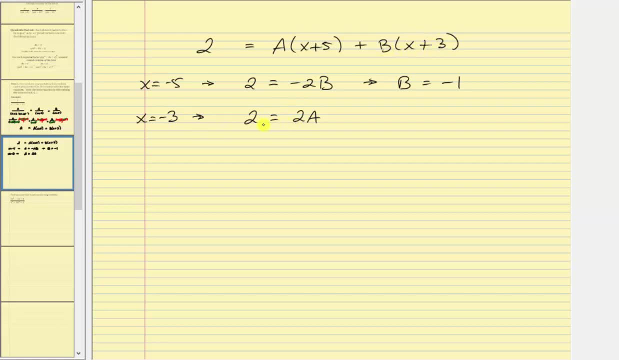 x plus three is zero. b times zero is zero, which gives us the equation two equals two, a. Dividing both sides by two, we have a equals one, And now we have the information we need to determine the partial fractions of the original rational expression. 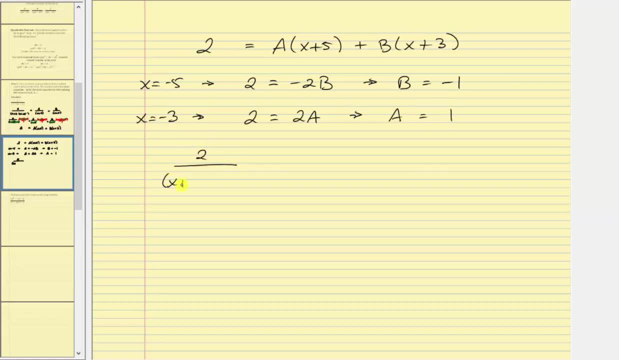 which was two divided by the product of the quantity x plus three and x plus five, which, remember we said, was equal to a divided by the quantity x plus three plus b divided by the quantity x plus five. And now that we have a and b, 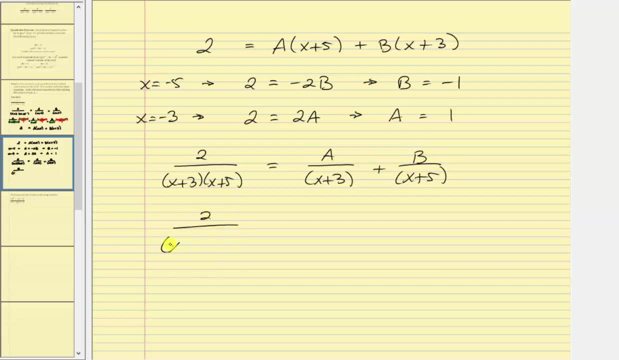 and now that we know a and b, we know the given rational expression is equal to a, which is one divided by the quantity x plus three. and then we have plus b, divided by the quantity x plus five, And since b is negative, one, 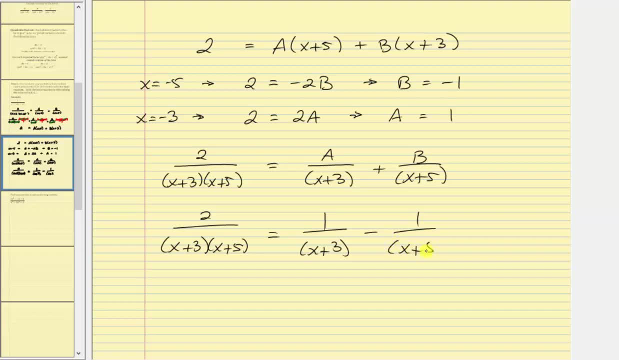 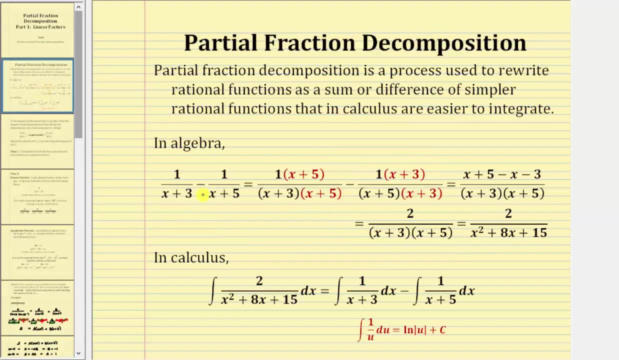 we can write that as minus one divided by the quantity x plus five. So this is the partial fraction decomposition of two divided by the product of the quantity x plus three and x plus five which, if we go back to the first slide, is verified from the difference shown here. 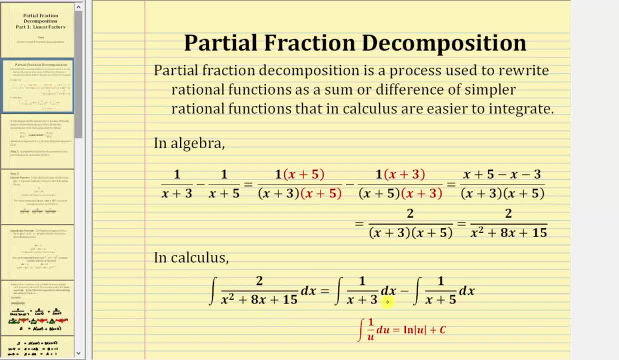 And again, the point of this is in calculus. if we have this integral, we can now find the difference of these two integrals, which is much easier to do using this basic integration formula. Let's look at one more example before we go. 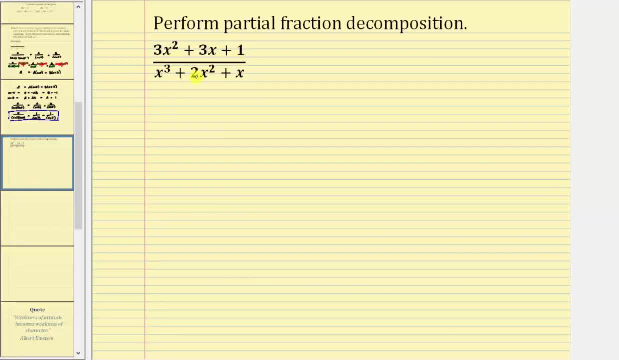 Let's determine the partial fraction decomposition of this, of this given rational expression. So again, first notice how the degree of the numerator is less than the degree of the denominator. So the next step is the factor of the denominator. The first step is to factor out the greatest common factor. 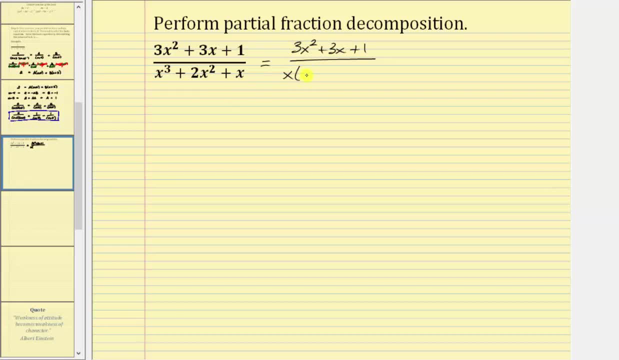 which is x. If we factor out x, we're left with the quantity x squared plus two, x plus one. And now we keep factoring. X squared plus two, x plus one will factor into two binomial factors. The factors of x squared are x and x. 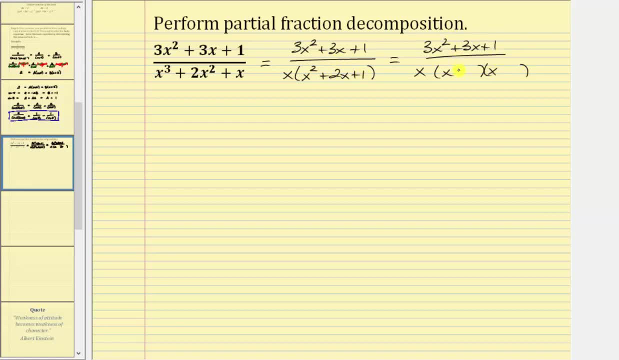 The factors of one that add to two are one and one, And therefore we have two factors of x plus one. So let's write this as: so. let's write this as the quantity three x squared plus three x plus one, And all this is divided by the product of x. 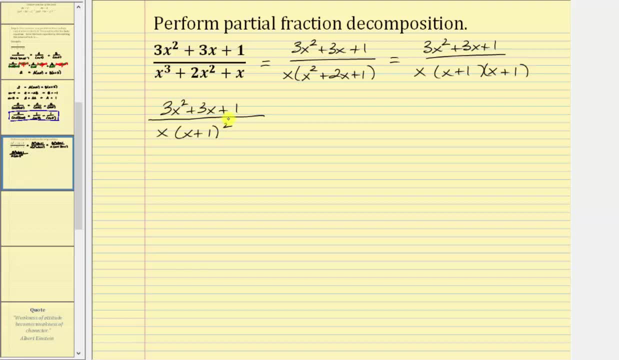 and the quantity x plus one squared, And now set up the partial fractions. X is a linear factor and therefore we have a divided by x and then plus we have the repeated factor of x plus one. So we have b divided by the quantity x plus one. 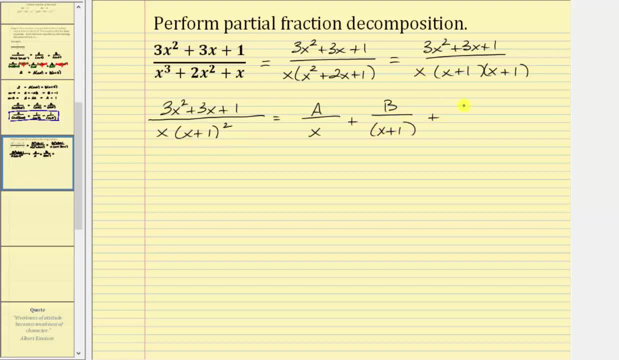 And then, because x plus one is a repeated factor, we also include plus c, divided by two factors of x plus one or the quantity x plus one squared. And now for the next step: we multiply every fraction in the equation by the least common denominator. 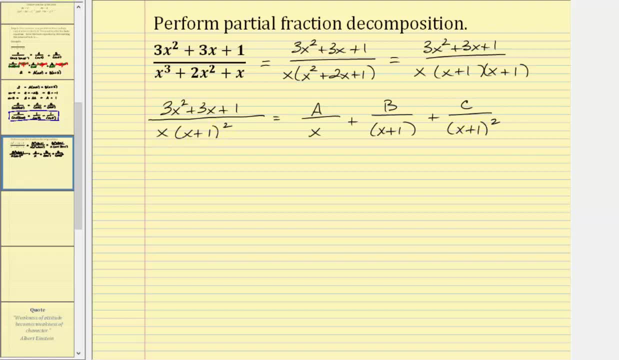 which is x times the quantity x plus one squared. So let's go ahead and set this up. Let's write x times the quantity x plus one, squared as a fraction with the denominator of one. And now we simplify before multiplying, Notice, here we have x divided by x. 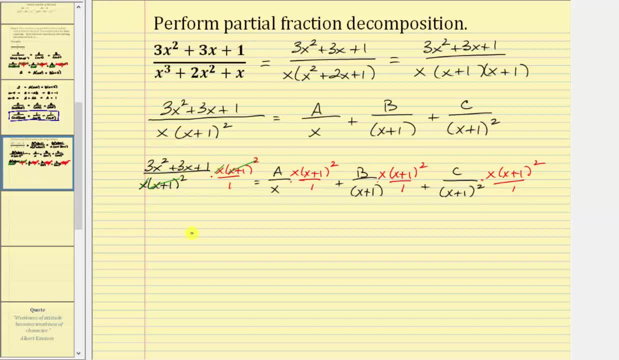 as well as the quantity x plus one squared divided by itself, leaving us with just three x squared plus three x plus one equals on the right side. here, only a factor of x simplifies out, leaving us with a times the quantity x plus one squared. 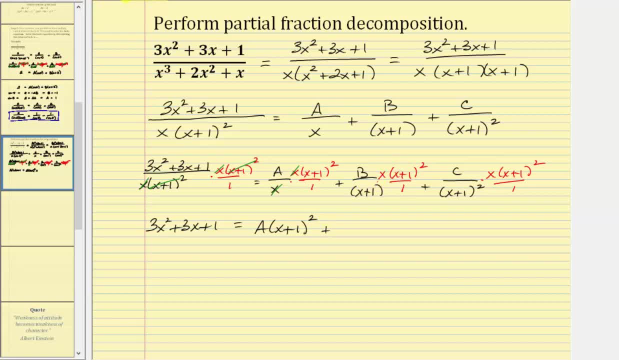 Then we have plus here only one factor of x plus one simplifies out. So this simplifies to one, that simplifies to one factor of x plus one, leaving us with bx times the quantity x plus one. And then here two factors of x plus one simplify out. 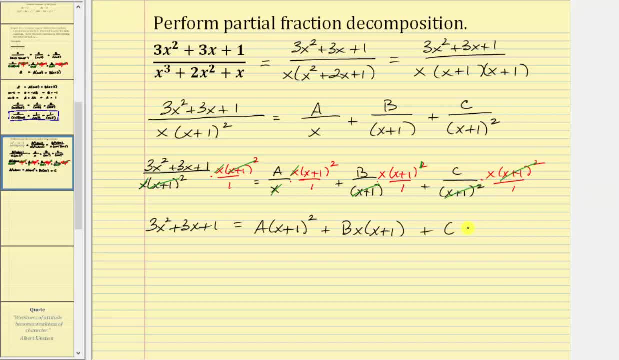 leaving us with c times, x or cx. So this is our basic equation, which you now need to solve for a, b and c, And let's do this on the next slide. And now, this equation is true for all the values of x. 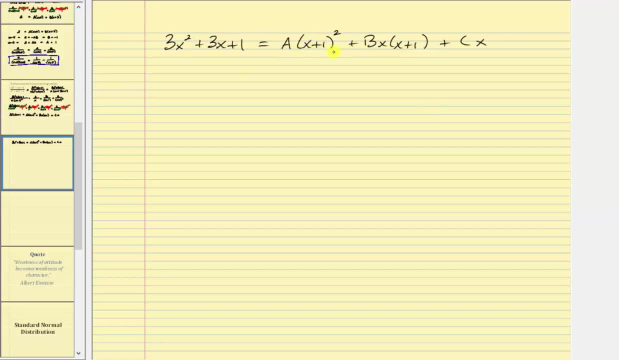 but again we'll select convenient values of x to make it easier to solve for a, b and c. We will let x equal zero and x equal negative one. Let's first let x equal negative one If x is negative one. 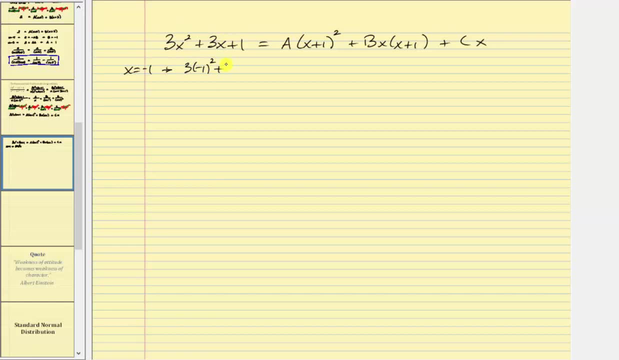 here we'd have three times the square of negative one plus three times negative. one plus one equals, if x is negative one, x plus one is zero here as well as here, leaving us with just c times negative one or negative c. So here we have three plus negative three. 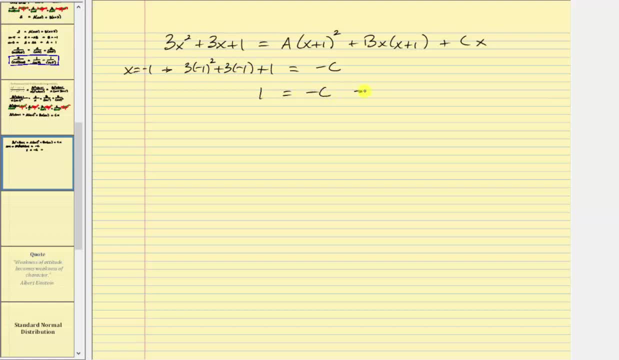 plus one, that's one. One equals negative c, and therefore c is equal to negative one. And now let's let x equal zero. When x is zero, we have zero plus zero plus one, which is one, equals on the right side. 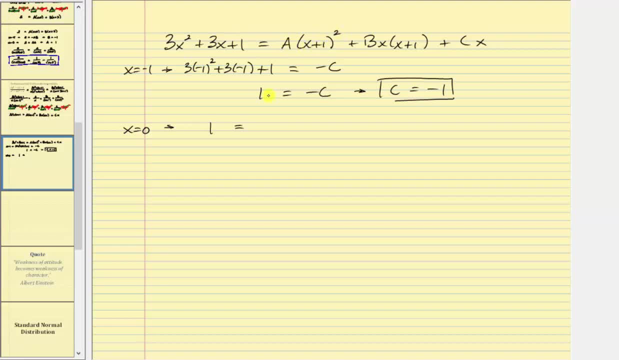 When x is zero, this would be a times the square of one, which is just a times one, or a. This would be zero, and this would be zero, and therefore a is equal to one. So now we know the values of a and c. 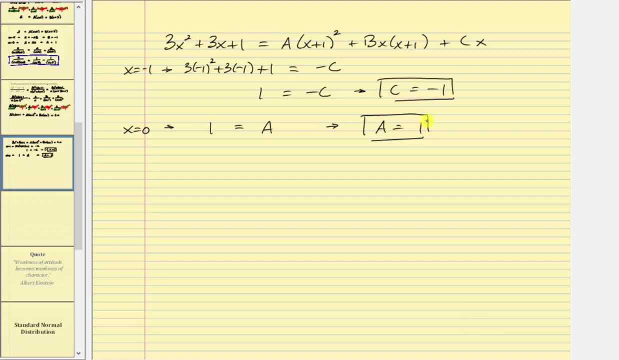 We just need to find the value of b, though, so we need to select another value of x. Let's try: x equals one When x is one on the right side. we have three times one squared plus three times one plus one, That's seven. 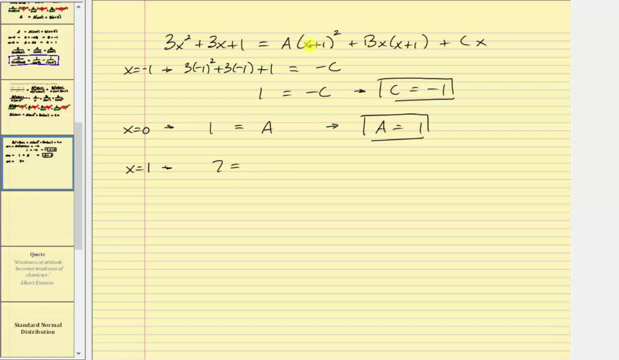 Equals when x is one. here we have the square of two, which is four. four times a is four a, but we know a is one, so we have four times a, which is one. so we have four times one plus.